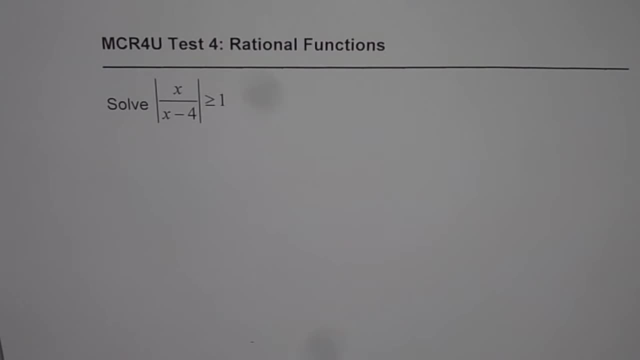 I'm Anil Kumar and here is an excellent thinking question for your test on rational functions, While some of my students are also having midterm and they need to go through this question carefully since it involves absolute functions and both rational functions and inequalities. Question here is: solve absolute value of x over x minus 4, greater than equal to 1.. 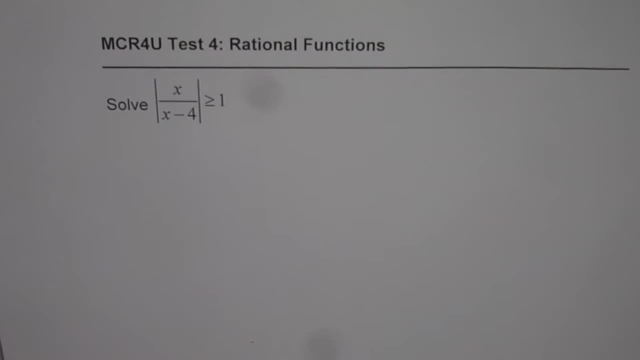 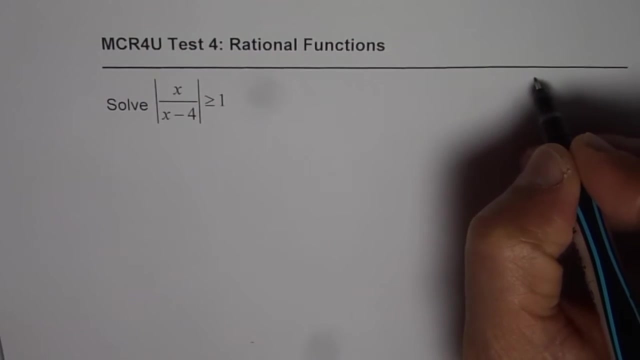 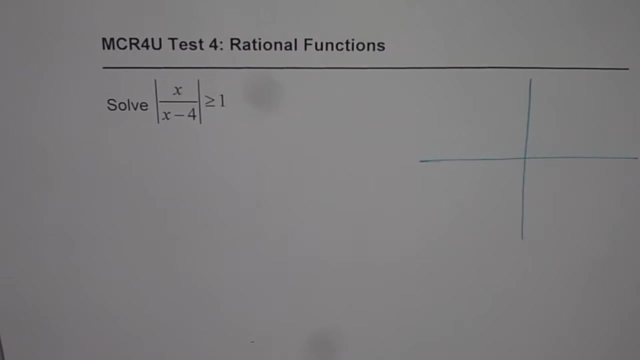 You can pause the video, answer the question and then look into my suggestion. Well, let's first analyze this function graphically and then we'll provide you with algebraic solution. So let us say that is the coordinate plane and we'll consider first the function x over x minus 4.. 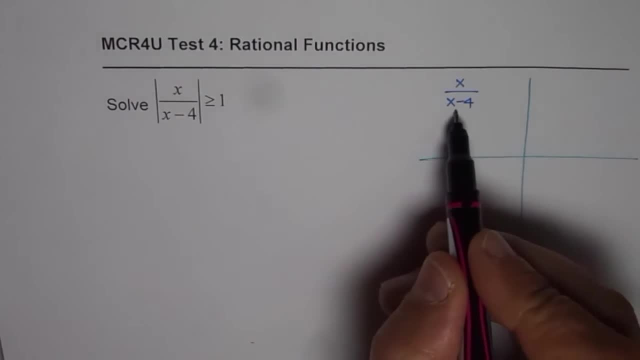 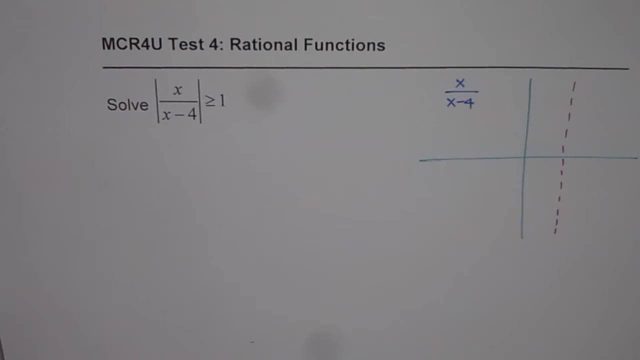 Now to sketch this function. vertical asymptote is at x equals to 4.. So I can draw a vertical asymptote like this, Which will be at x equals to 4. And the horizontal asymptote is going to be at 1, right. 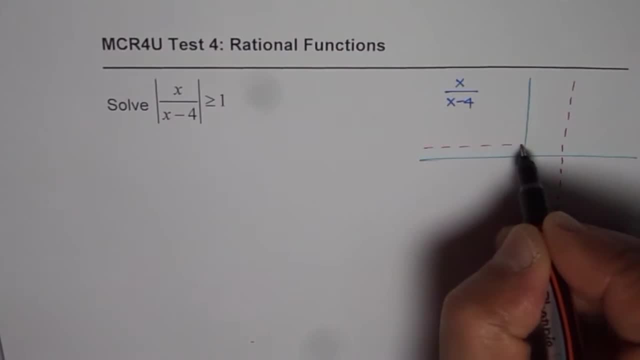 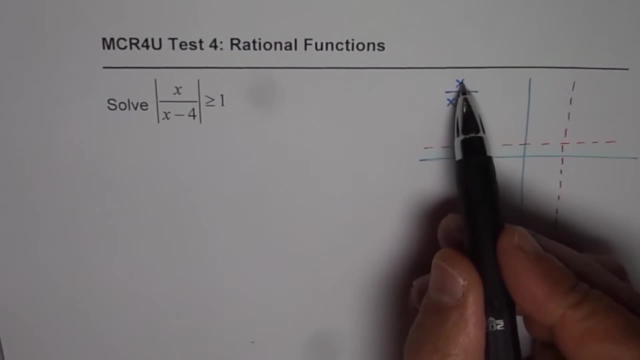 x over x, which will be at 1.. So let's say this is the horizontal asymptote at 1.. And what is the xy intercept When x is equal to 0, then we get 0. That means y intercept is at 0.. 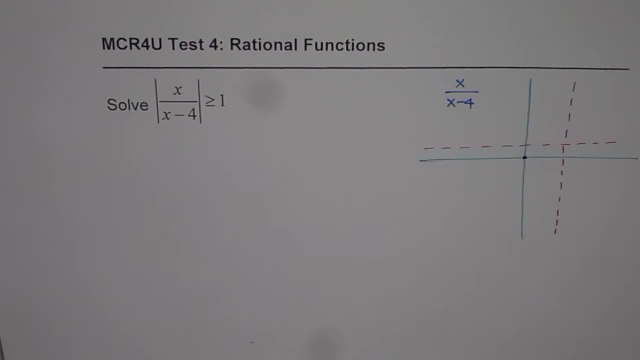 Now that helps us to sketch the graph. So I'll quickly sketch the graph from these points. We know horizontal asymptote, Asymptote going through the intercept, So it is symmetric about this point. So it has to be like this: 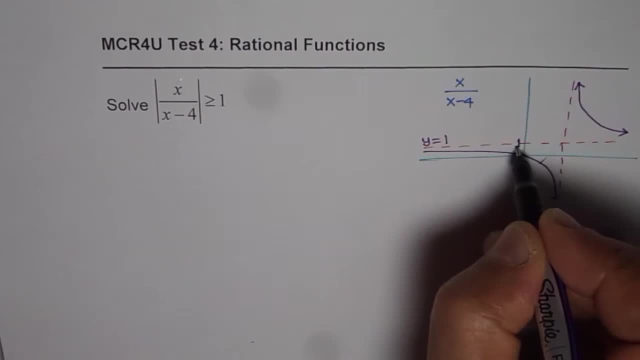 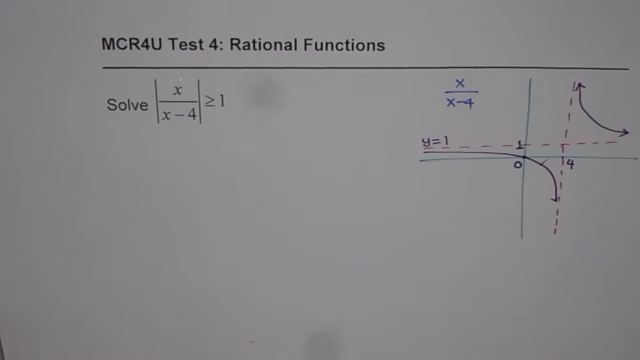 So we have y equals to 1.. So this value is 1 for us, And this value is 4 for us. Here we have a 0. Now what is absolute value of this function? So this rational function, if I say absolute value. 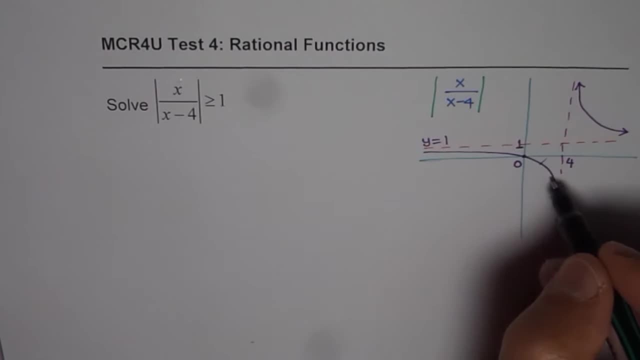 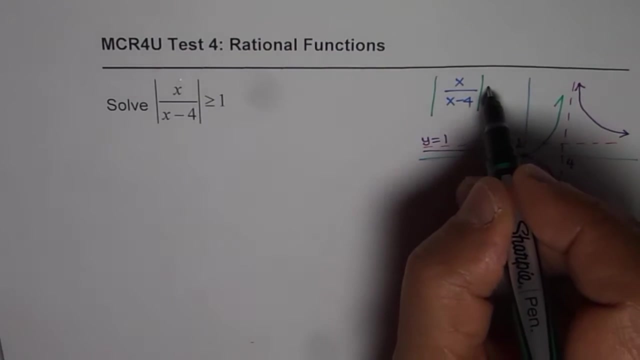 then the negative part becomes positive, So this portion which is negative gets reflected, correct. It's kind of like this: Now we have to solve the inequality greater than equal to 1. So the solution is very clear before us, correct? 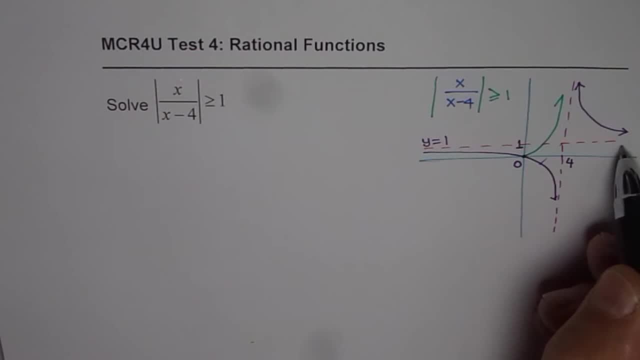 The solution, of course, one part is: whenever it is greater than 4, the absolute value will be positive, But also when this point is that okay, That is, when the function is minus 1, afterwards between minus this x value. 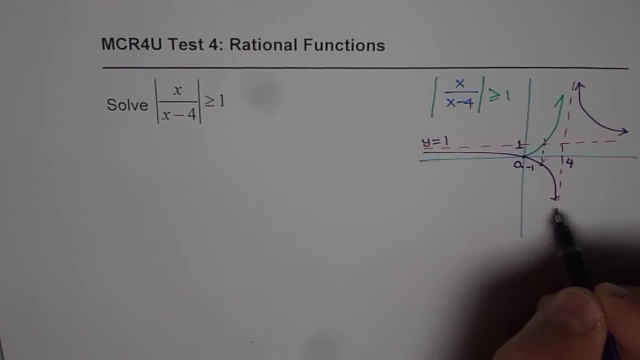 whenever it is minus 1, will also lead to the solution right. So we need to find the x value when the function is minus 1 to get to this part of the solution, right. That is one way of looking into it. 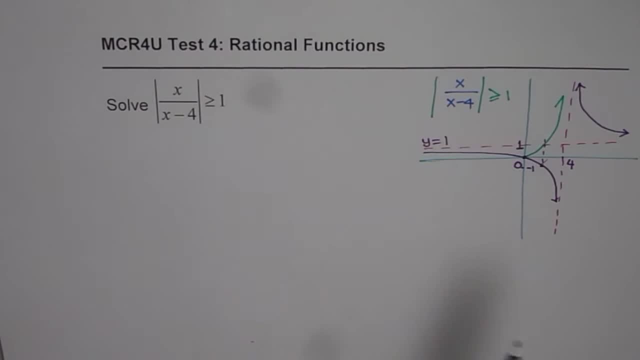 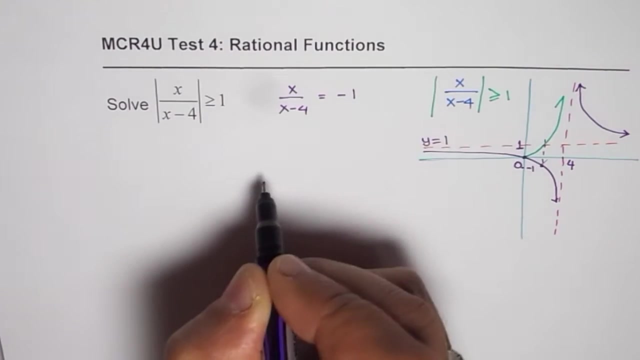 So you can definitely solve this inequality as such And that is a good approach to see. So let me do a shortcut method, That is, we will solve for this function which is x over x minus 4 equals to minus 1.. 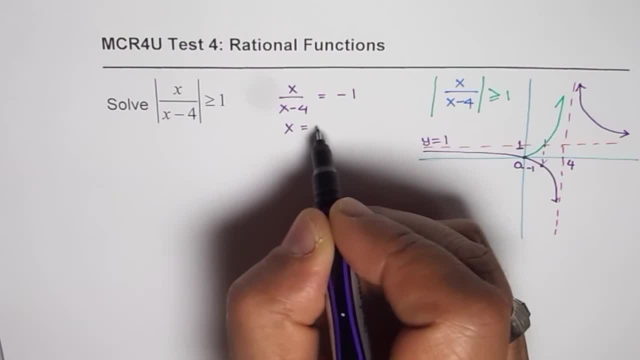 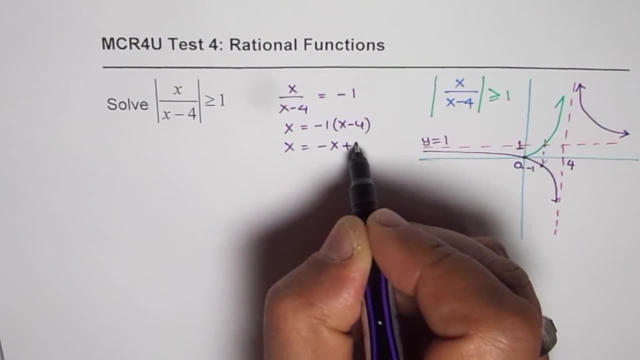 So if we solve, we get x equals to. we'll cross multiply, which will say minus 1 times x minus 4.. So we get x equals to minus x plus 4.. So we'll bring it here: So we get 2x equals to 4,. 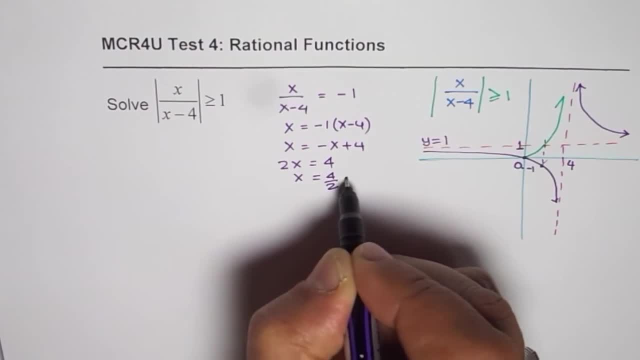 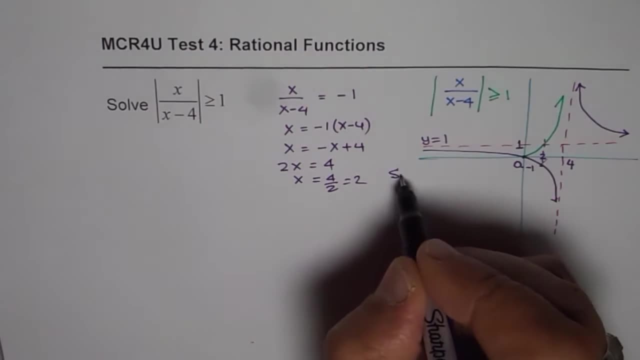 or x, is equals to 4 divided by 2, which is 2.. So this point is 2.. Since this point is 2, we have our solution, And our solution is: from 2 to 4, correct, greater than equal to. 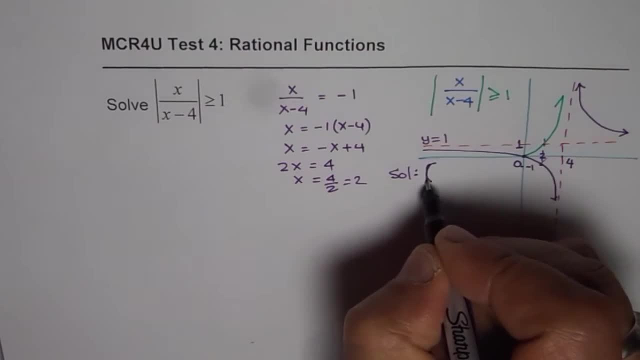 you could include 2, because it is equal to right. So we'll include 2,, correct from 2,, but 4 is not in the domain, So 2 to 4, not included. Union 4 is not included. 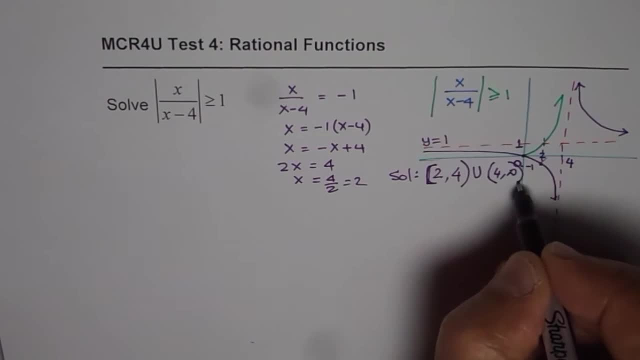 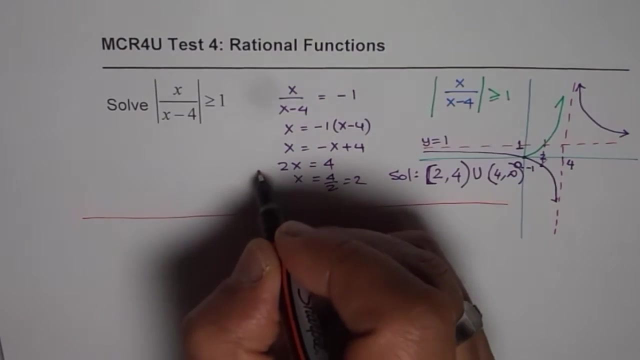 since it is a vertical asymptote to infinity. Do you see that? So that becomes our solution Correct. So that's a fast way of doing and understanding this question. The alternate way to do this is whenever we are working on absolute function. 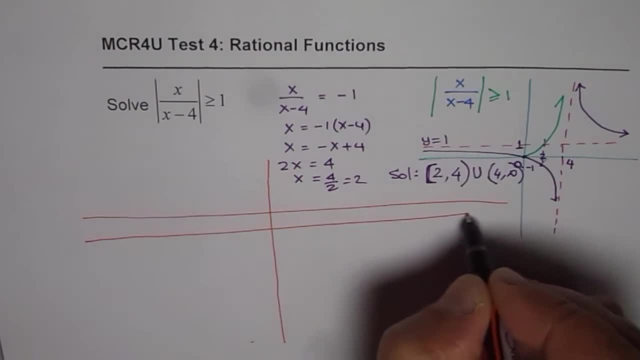 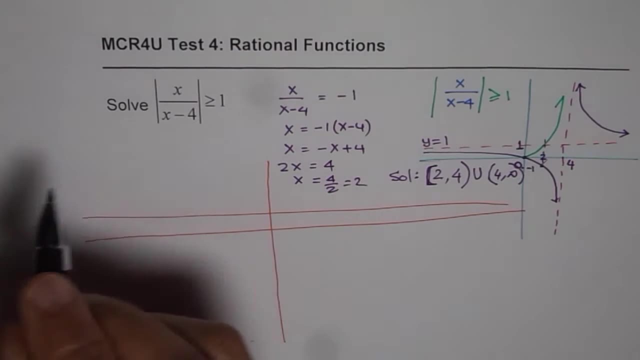 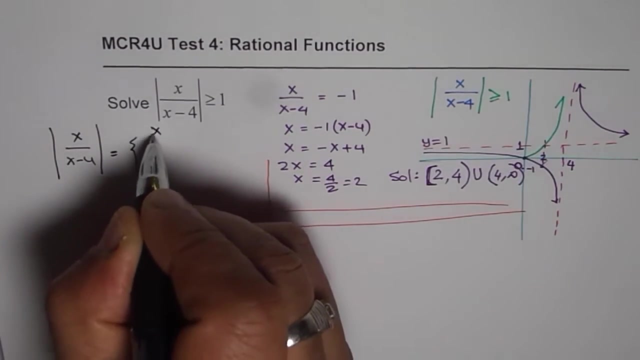 you have to do it in two domains: One when the function is positive, The other when the function is negative. right, Since this value of absolute function- x over x minus 4, absolute value can be defined as x over x minus 4,. 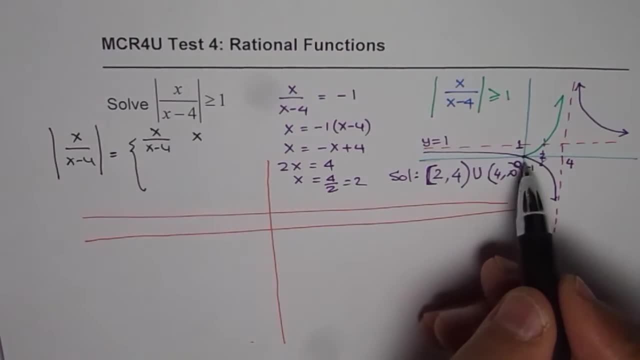 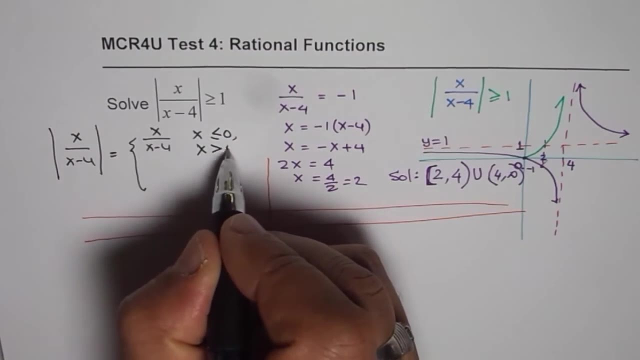 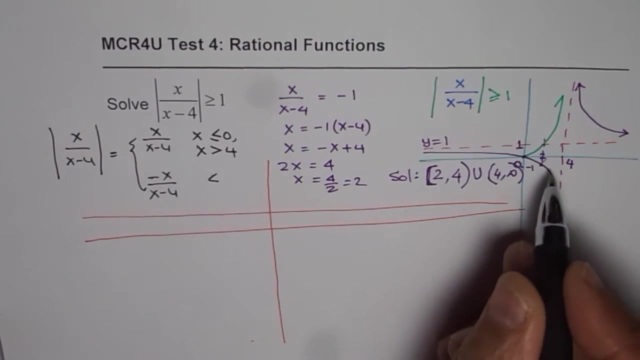 if x is less than 0, right. If less than you can say less than equal to 0, or if x is greater than 4, is it okay. But it is negative of this value when x is greater than 0,. 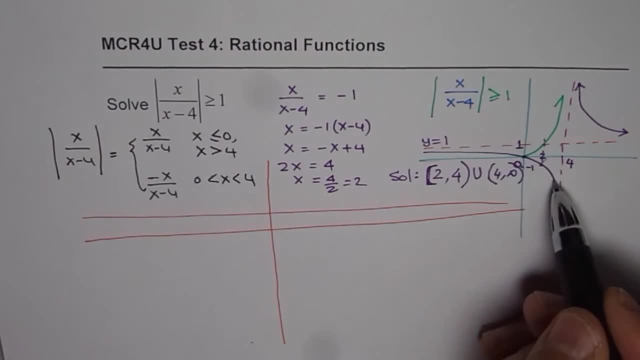 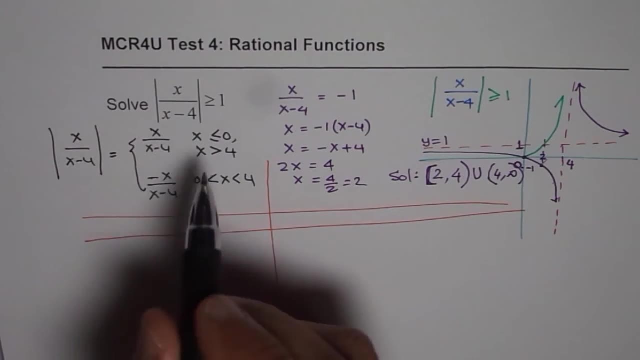 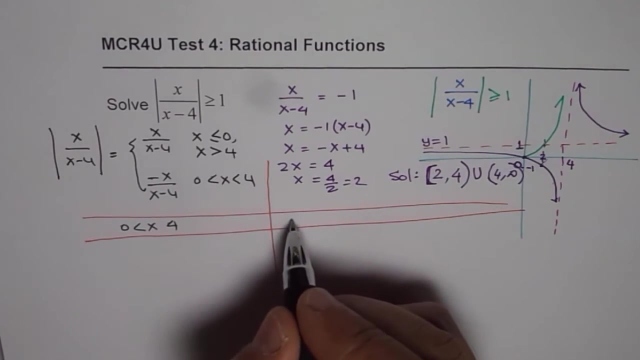 but less than 4, correct, Since absolute value will reverse. So that is how the function is. So we need to solve this within these two groups, correct? So let's solve for x between 0 and 4, and for x when x is less than 4,. 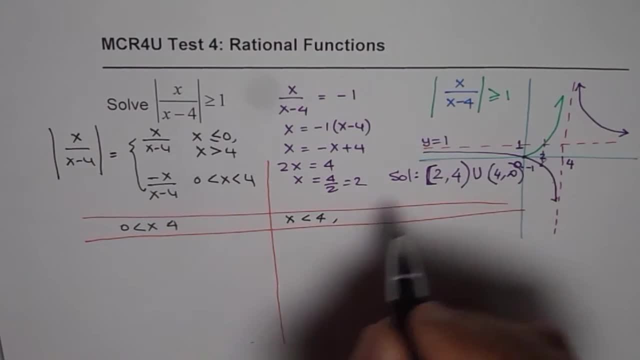 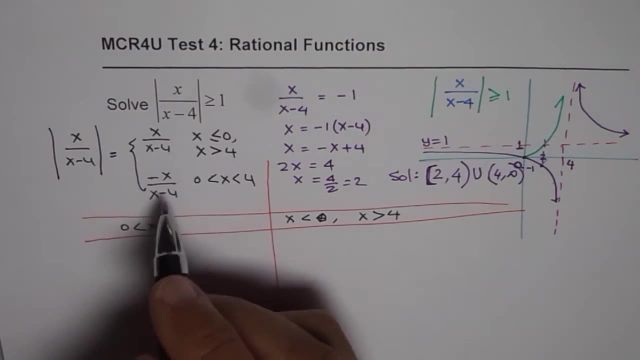 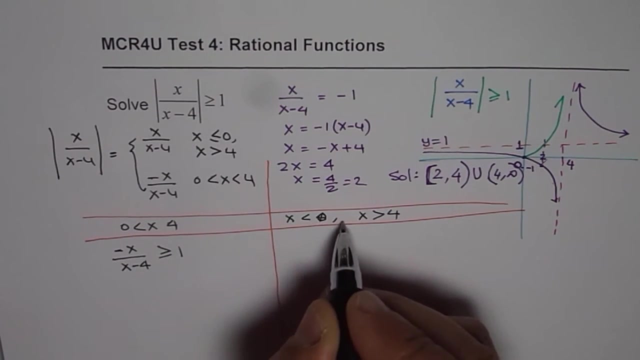 or I mean less than 0, or x is greater than 4,, correct. In this case, your inequality will be minus x over x minus 4, greater than equal to 1, and here the inequality will be. 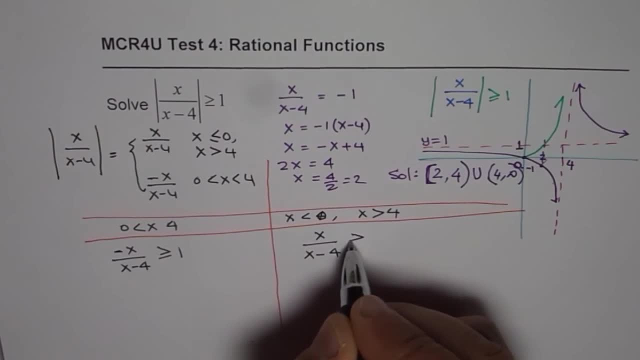 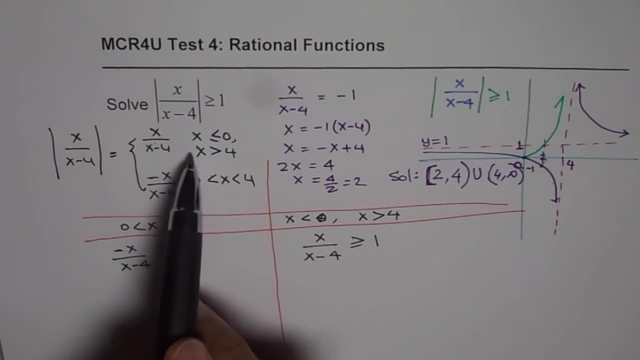 x over x minus 4, greater than equal to 1.. Do you get the point? Since absolute value is defined like this? So within this interval it is positive And in this interval it is negative of that value, Correct? 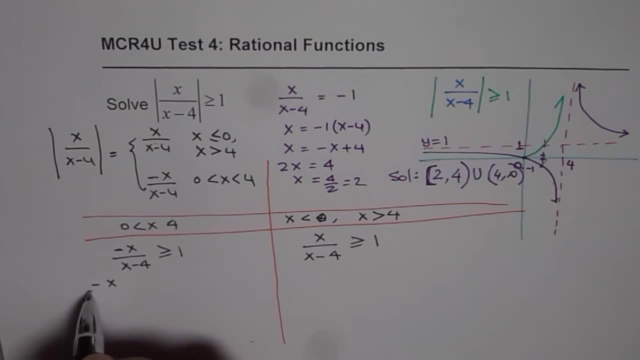 So now you can bring 1 to the left side, so we have minus x over x minus 4, minus 1, greater than equal to 0, take common denominator which is x minus 4, minus x. when you multiply you get minus x plus 4,. 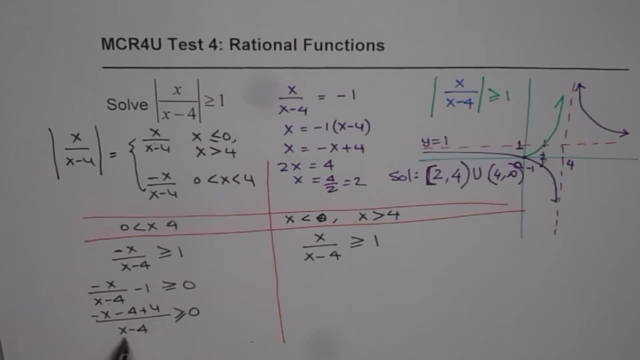 greater than equal to 0. And when you solve this and similarly this side, also same thing, you'll do x over x minus 4 minus 1, greater than equal to 0, x minus x minus 4, when multiplied it becomes plus 4,. 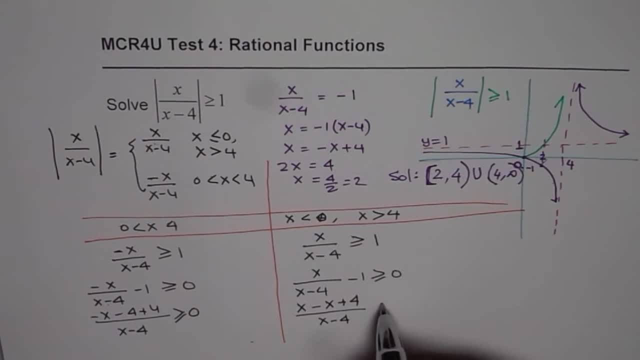 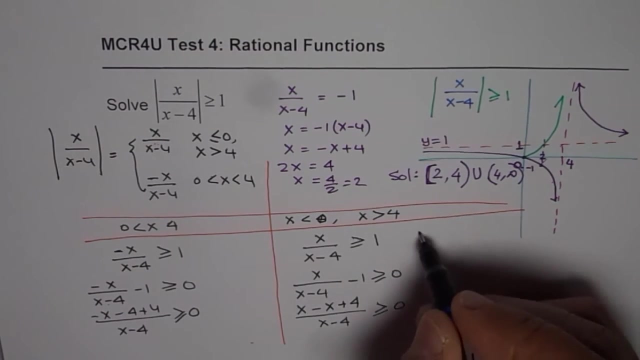 and here you get x minus 4, greater than equal to 0. Correct Now, which is which is this becomes 0, so we are running out of space, so let me just divide it and move it further. 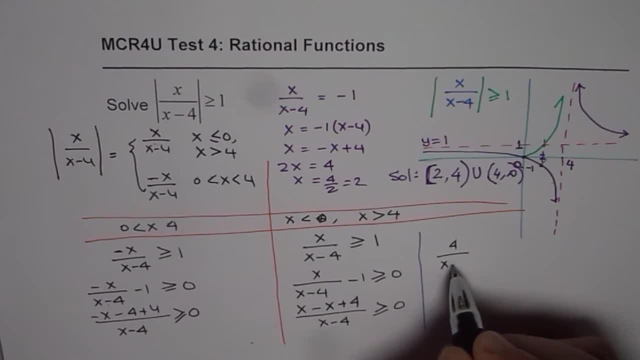 so it becomes 4 over x minus 4, is greater than equal to 0.. Correct Now: if x is greater than 4, then 4 over x minus 4, will be positive. so it is always true. 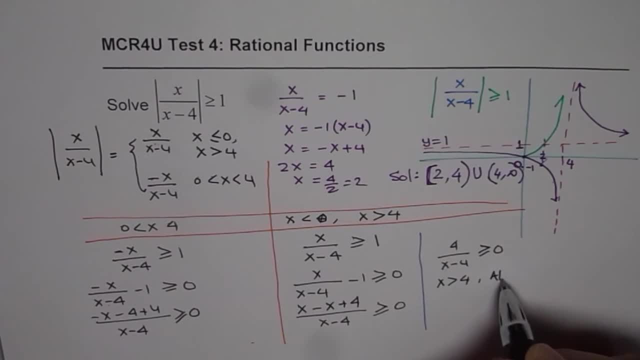 So if, if x is greater than 4, it is always true, Is that okay? So we get this part of our solution, but if x is less than 4, I mean less than 0, this is 0 for us. 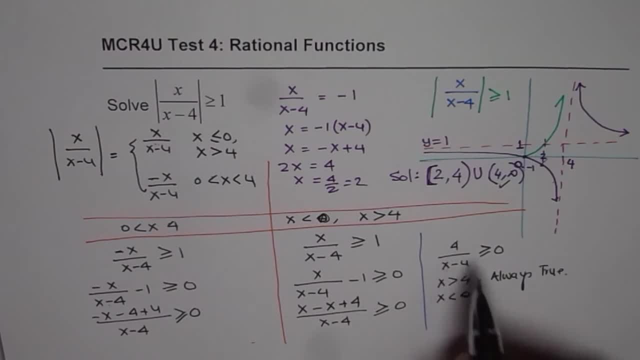 less than 0, that means it is negative. then this value will be negative. it is never true. So the solution from here we get is when x is greater than 4, it is that part of the solution. Now we can solve this one. 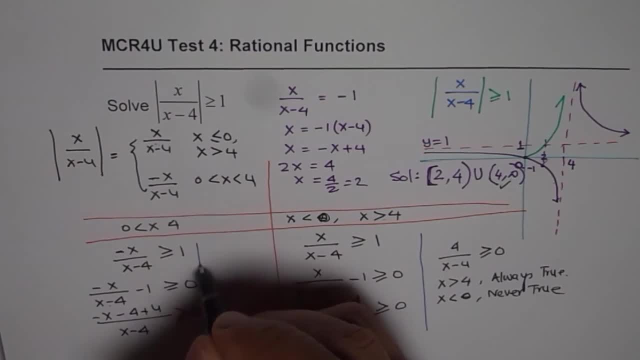 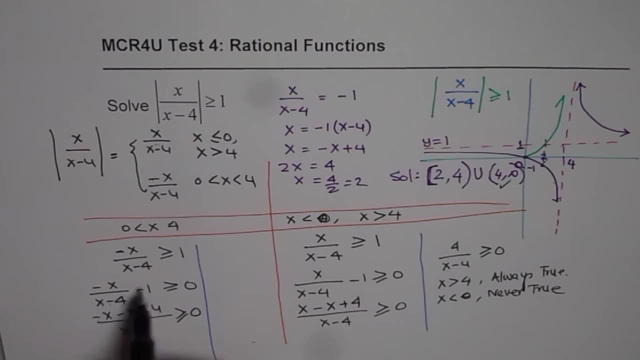 which gives us. okay, let me also break this. so we get: so this is minus x, sorry. so you multiply minus x plus 4, so you get minus 2x plus 4, over x minus 4,. 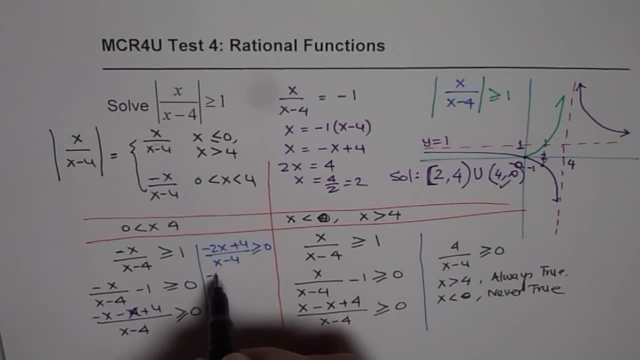 is greater than equal to 0, we can take 2 common. let's take minus 2 common, x minus 2, over x minus 4, greater than equal to 0, so that gives us 2 zeros, right. 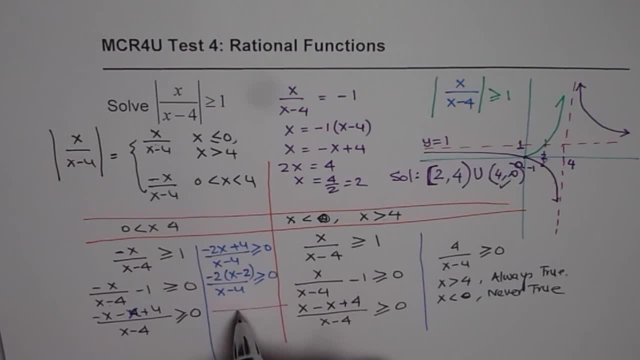 Let's analyze this portion. the 2 zeros are at: x equals to 2, and x equals to 4,. x equals to 2, and x equals to 4,. right, And if you have test points, let us take a test point. 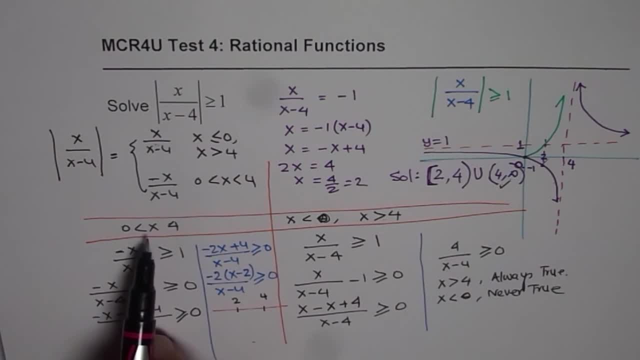 on the left side it could be between 0 and 4 only, right. So we can take 1 and 3 here, correct? So if I take a test point 1,, for example, then my question will be: 1 minus 4 is negative. 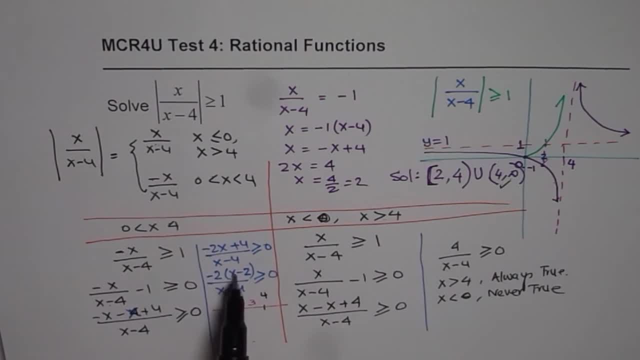 and here 1 minus 2 is minus 1, times minus 2 is positive, so we get negative, so this value is negative. if I substitute 3 here, then what do I get? I get: 3 minus 2 is 1,. 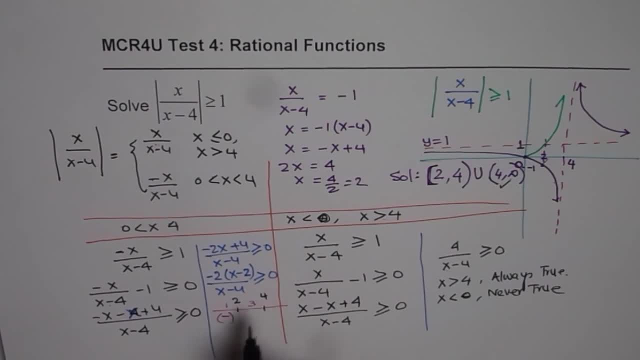 1 times minus 2 is minus and this is minus 1, so we get plus answer here. so we get that as positive. therefore, this interval is a solution correct. So we get our solution as. let me push the page. 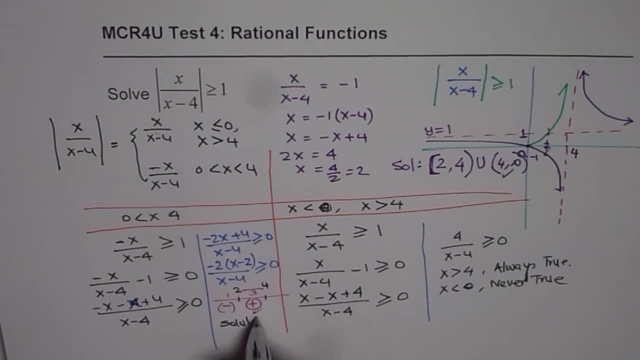 so from here we get the solution, as x is between 2, because it is equality and equal to right. So it is: x is greater than equal to 2, but less than 4, that is one part.